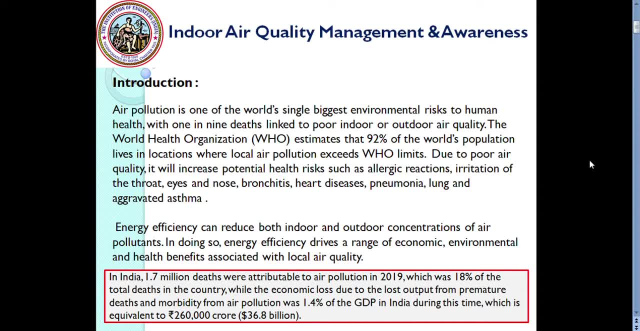 And WHO estimated that 92% of world population lives in the location where the local air pollution exceed WHO limits And, due to pure health quality, it will increase potential health risks such as allergies reaction, irritation of the throat, eyes and nose munches, heart disease. 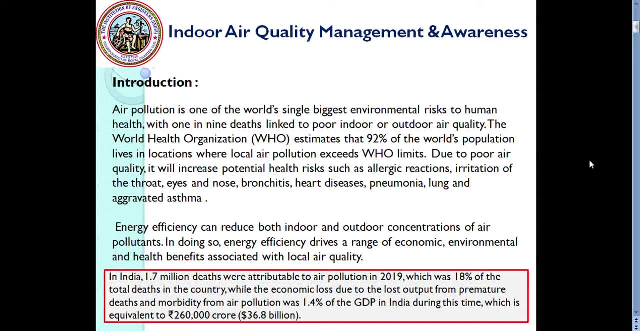 pneumonia, lung and aggravated asthma, But energy efficiency can reduce both indoor and outdoor concentration of air pollutants. In doing so, energy efficiency drives a range of economical, environmental and health benefit Associated with the local air quality, And in India over 1.7 million deaths were attributed. 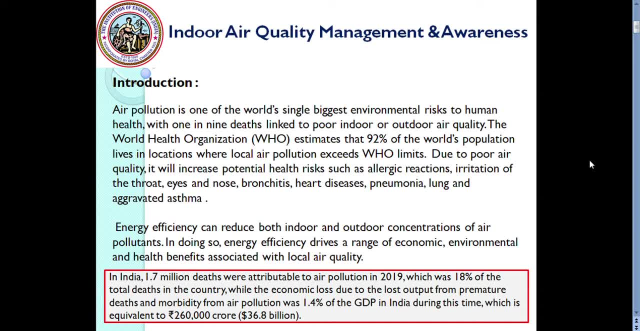 to air pollution in 2019, which was 18% of the total in the country, While the economic losses due to the output of the premature death and vulnerability from the air pollution was 1.4% of GDP in India during this time, which is equivalent to 250,000 crore, which is used. 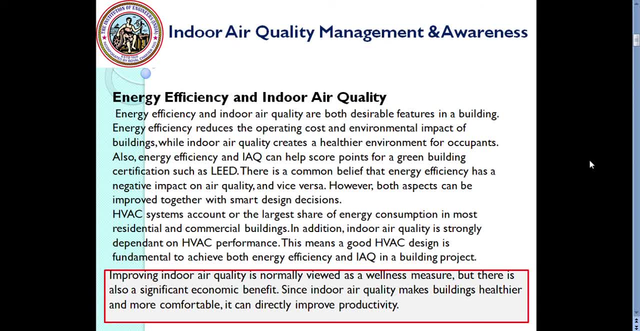 Energy Efficiency and the Air Quality. Energy efficiency and air quality: both are desirable feature in the building or commercial spaces, And energy efficiency reduce the operating cost and environmental impact of the building, while indoor air quality creates a healthier environment for occupants. Also, energy efficiency and the air quality can help source score point for the greener building certification. 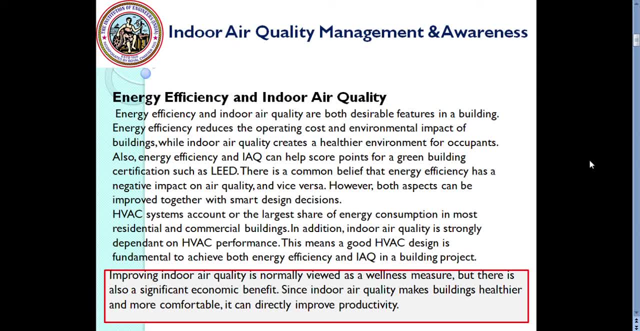 There is a common belief that energy efficiency has a negative impact on the air quality and vice versa. However, both aspects can be improved together with a smart design decision. and heat ventilation air conditioning system account or the largest share of energy consumption in the most of residential and commercial building. In addition, 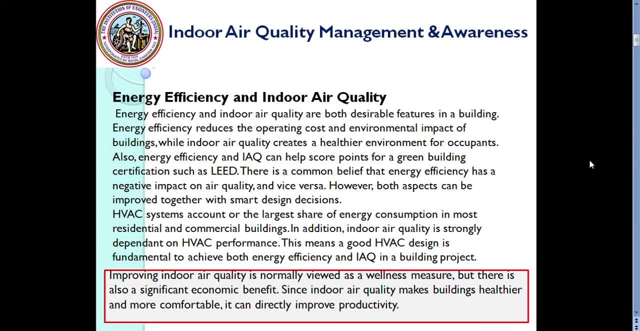 indoor air quality is strongly dependent upon HVAC performance. This means a good HVAC design is fundamental to achieve both energy efficiency and indoor air quality in the building projects. Improving indoor air quality is normally views as a wellness measure, but there is also a significant economic benefit, Since indoor air quality makes building healthier and more comfortable it can. 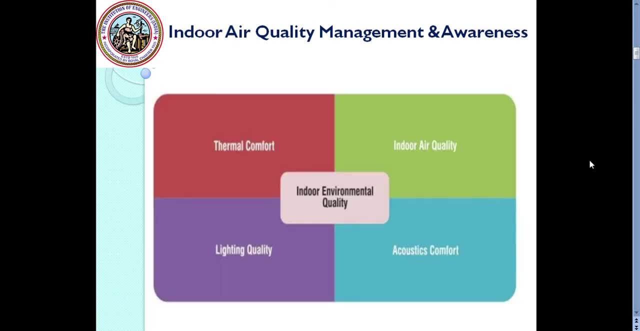 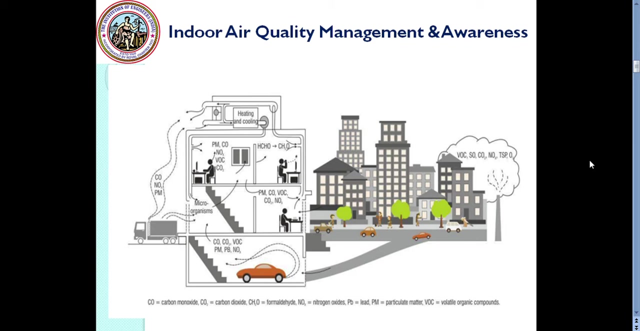 directly improve productivity. This is just a kind of indoor air quality, environmental where we consider thermal comfort, indoor air quality, lightning quality and acoustic comfort. Overall is indoor environmental quality. This is just a kind of indoor air quality that is designed to be sustainable, In addition to its low pollution. 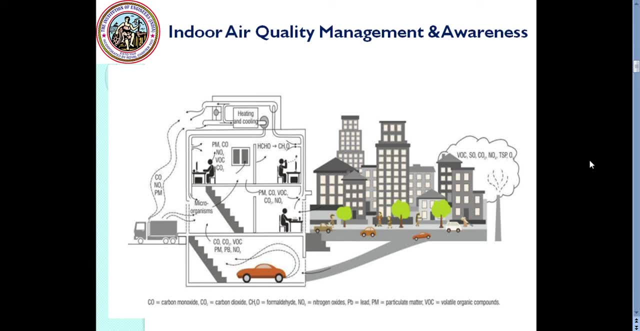 which goes from outside to inside, and how this pollution ventilate Over there. we can see from the transport which is for the carbon monoxide, nitrogen, sulfur particular matter and this with the heating and ventilation it goes to the over spaces and some of the industry where it is always. 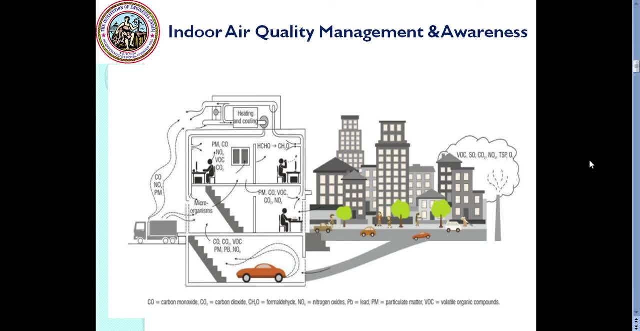 some kind of manufacturing process is going on. A lot of components generated within the unit and we are discussing the same process for the other components. There is a number of different generate inside which has to be eliminated to make the environment comfortable and healthier, such as the voltaic organic compound, particular matter, nitrogen oxide for 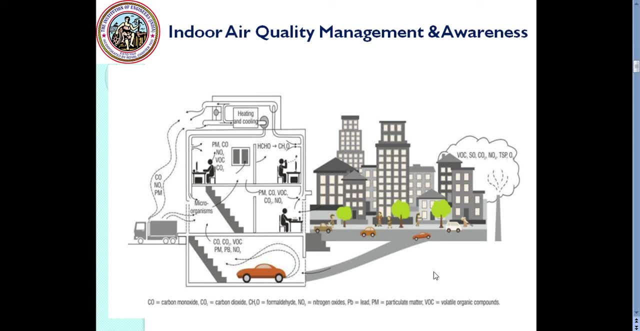 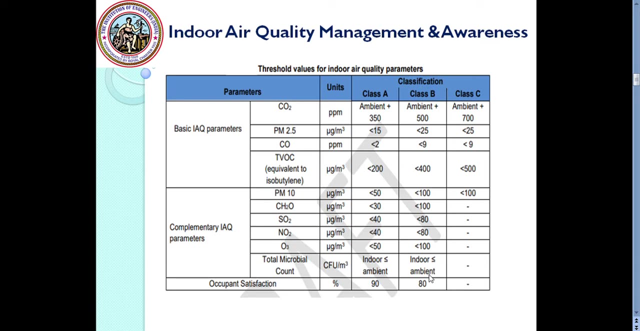 might. so these are the things which can generate in the industrial, environmental and which has to taken care very consciously to maintain the indoor air quality from the indian associations. we don't have any indoor air quality standard on the national level but icera has developed some indoor air quality parameters which is having some 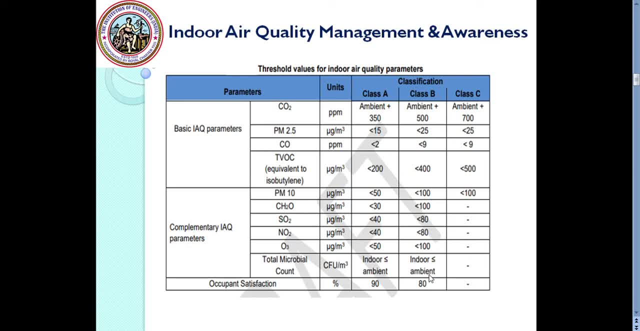 basic indoor air quality parameters like carbon dioxide, particular matter 2.5, carbon monothese and isobutane, and there are some complementary parameters which we can see in the figure and this classification has been in the class a, class b, class b which we will evaluate in the coming slides. 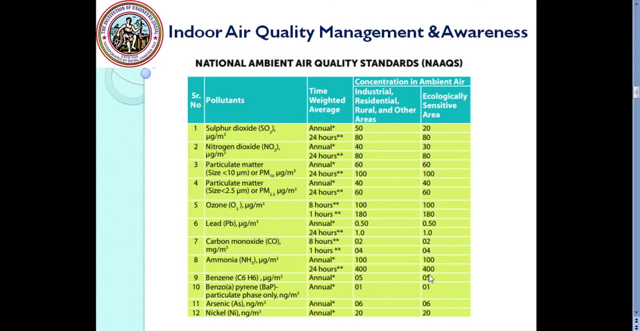 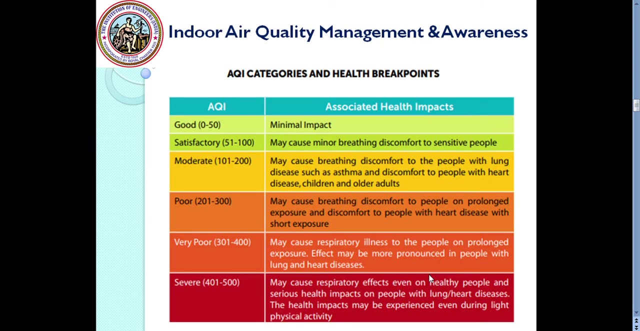 but we do have national ambient air quality standard for outside and these are the parameters which is given for the industrial, residential cooler and other areas and some of the air quality index which gives which kind of the environmental we are living and these are the figures which give the 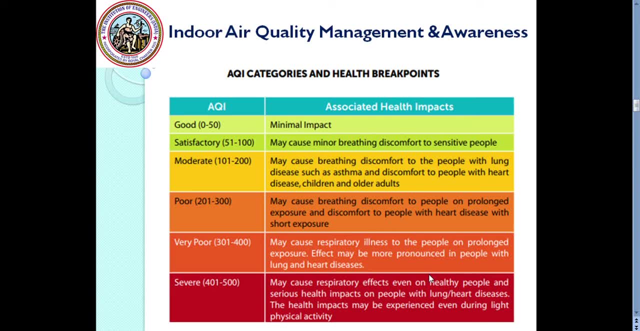 index. if it is 0 to 50 it is good, 51, 200 satisfactory. 100 1 to 200 is moderate, 200 to 300 poor and 300 to 400 very poor and 400 to 500 very severe. what are the very, you know, benefits we are? 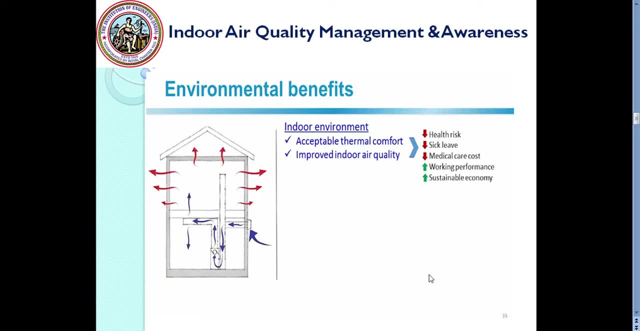 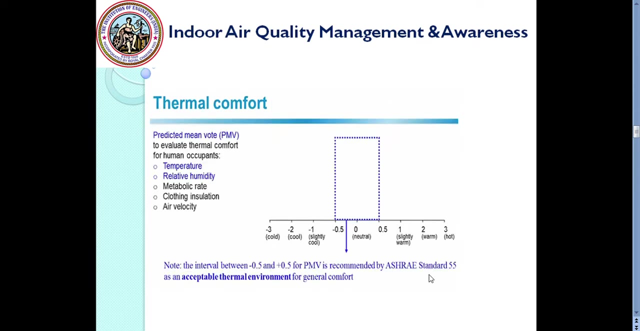 getting from the indoor air quality like it it gives if it is our industrial area. it reduces the health risk. do the silk leaf medical care cost and improve the working performance and sustainability economy. these are some parameters which gives the thermal comfort, like temperature, relative humidity, metabolic rate, clothing insulation, air velocity. this is a from the ashray standard. 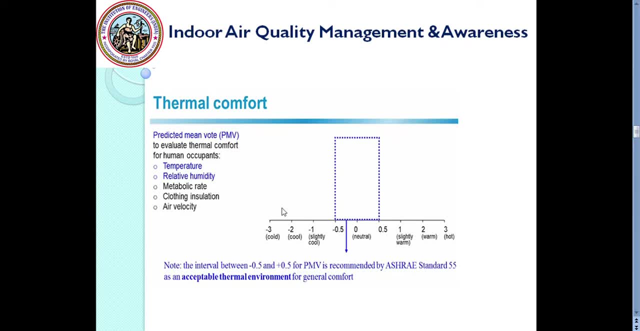 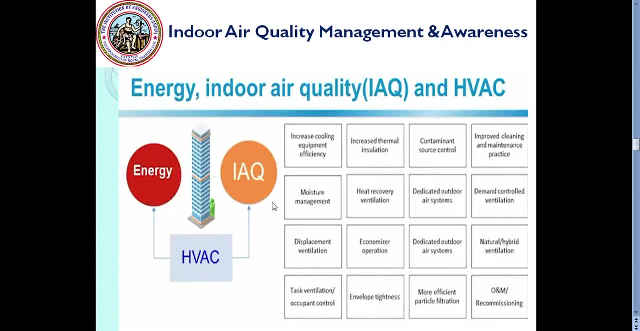 and this is a point we are saying: this is acceptable. thermal, environmental for the general comfort, energy, indoor air quality and the heat ventilation, air conditioning depend upon the lot of various parameters there are, like what kind of equipment, what are the efficiency we have, what kind of insulation we have, what kind of the contaminated source we are getting in our environmental indoor. 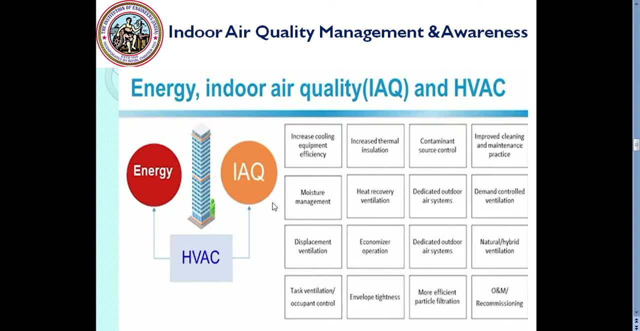 What are our cleaning and maintenance practices? Moisture management, heat recovery, ventilation. dedicated outdoor air system, demand control, ventilation displacement, ventilation economizer operation. dedicated outdoor air system, natural hybrid ventilation, task ventilation envelope tightness, more efficient particle filtration. operation and maintenance and reconnectioning. 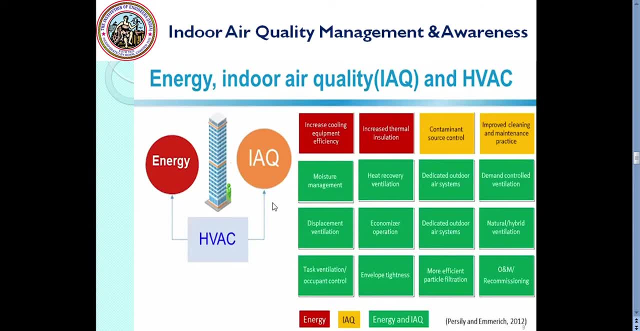 So if we consider how these are the relevant to the energy, indoor air quality and the heat and ventilation and air conditionings. So if we see this red color, it is dedicated to the energy, like the cooling and heating effect from the equipment. If equipment are more efficient, more energy efficient, obviously it will draw less energy. 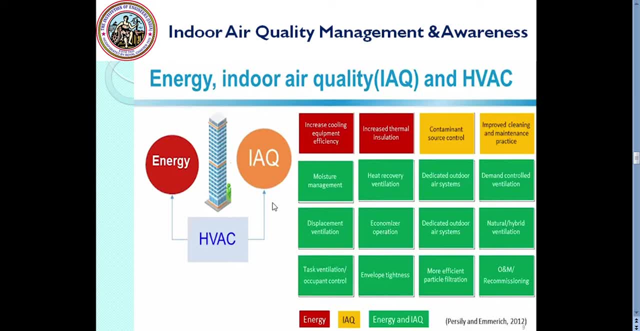 Increased thermal insulation which will keep the environmental in more time to the maintained temperature, so it will reduce the energy consumption. So this particular two red tabs are directly associated with the energy and the contaminated source control and improved cleaning and maintenance practices directly associated with the indoor air quality. 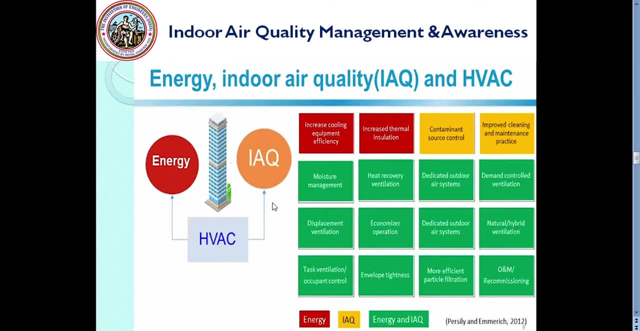 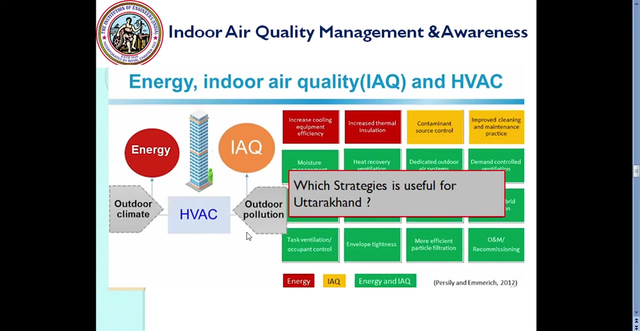 Other parameters- moisture management, heat and recovery, etc. are directly related to the energy and the indoor air quality. This is the same for both But it depends upon, like now, how our outdoor climate is there, What are the outdoor pollution? So it depends upon the location: what are the scenarios of the pollution and what is the climate, So we can define what kind of a strategy will be useful for the our state, Uttarakhand. 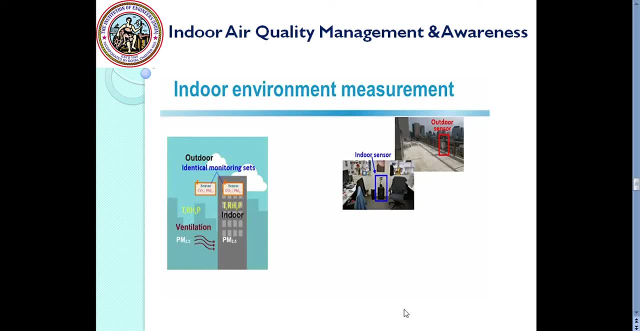 So this is just one kind of the assumptions. taking the high-rise building over there we have the indoor and outdoor sensor and this is a continuously monitoring of what kind of the pollution outside and indoor. so with the indoor sensors they are giving the command and accordingly the ventilation or demand ventilation. 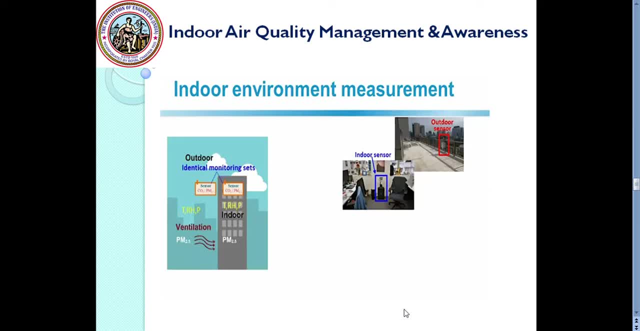 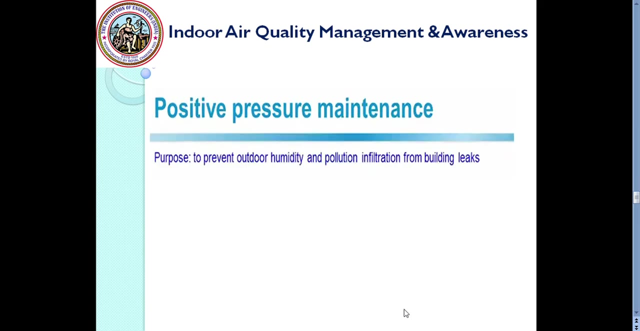 open or close more air intake. all those parameters has been controlled with the controller and maintain the adequate thermal comfort and the air supply. and we have to always maintain the positive pressure inside the premises so that it will prevent the outdoor humidity and the pollution infiltration from the building leaks. and with the building management system with a smart 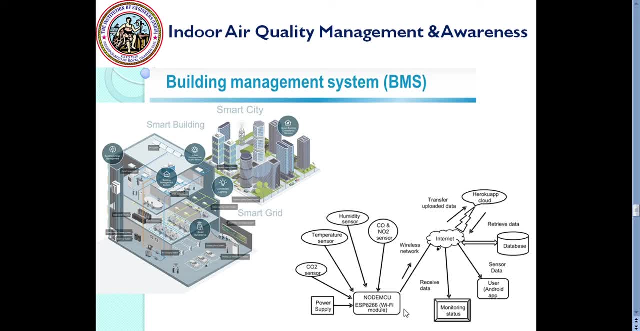 building, we can control a lot of things and energy can be efficiently managed and with the real-time monitoring of the various gases- temperature sensors, humidity, a lot of the parameters are getting the real-time information about these from these sensors to maintain the real status, and it very efficiently and it will. with the low energy consumption, the comfort can be. 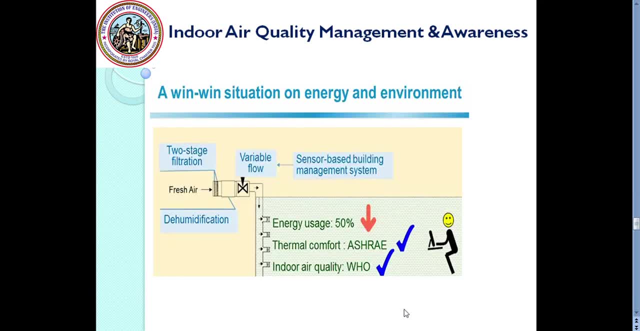 maintained, the indoor air quality can be maintained. so this is this kind of the layout figure: how, with the good ventilation and good real-time air monitoring uh, it will be win-win situation for both in their air quality and the energy consumptions. with a good design we can achieve almost 50 percent.